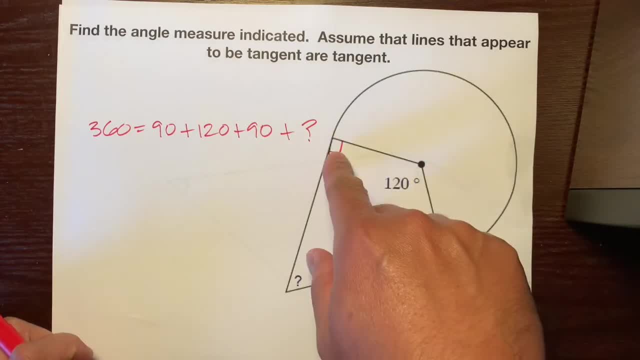 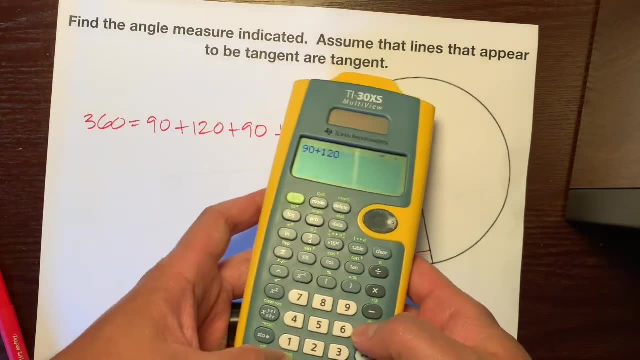 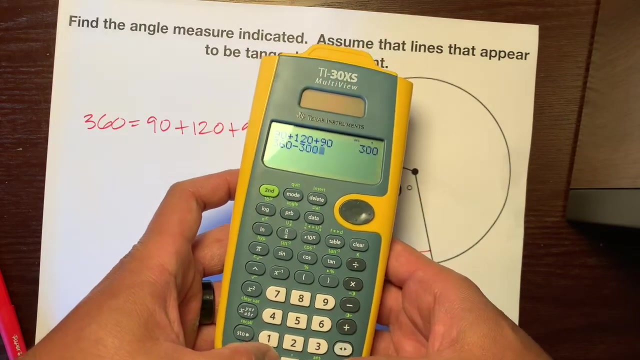 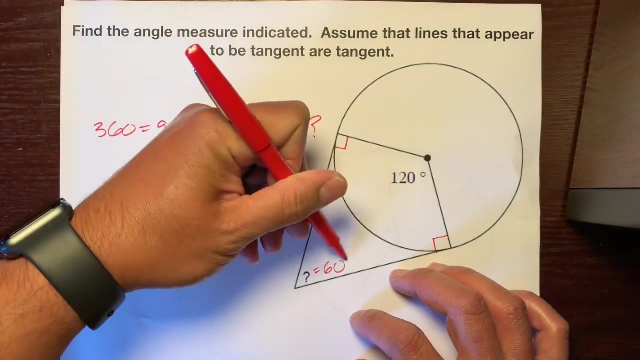 and let's just keyboard select the bottom figure and 66 degrees and subtract that. So where do these sides Milli? They're somewhere aroundountain 220 or more. So I'm limited by my рис snack and I create that space, So I'll just go ahead and sort. So let's say 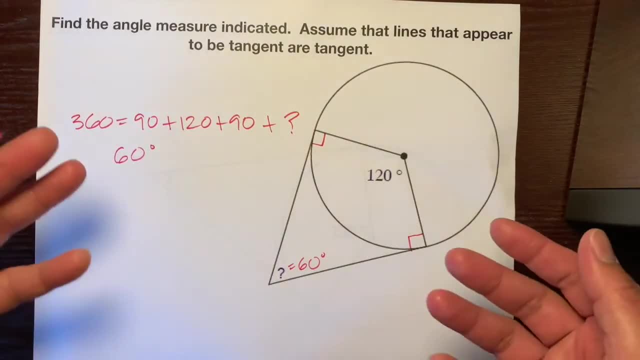 that minus었다's a nine plus one, So I'm going to do this by subtracting this one from my minus었다's, If your teachers taught you this yet. so, because this is a 120 degree angle, this is if you've. 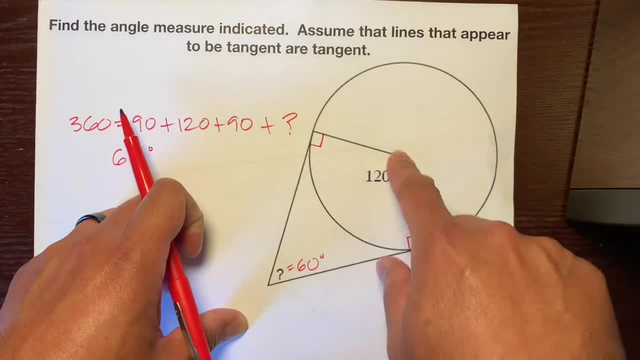 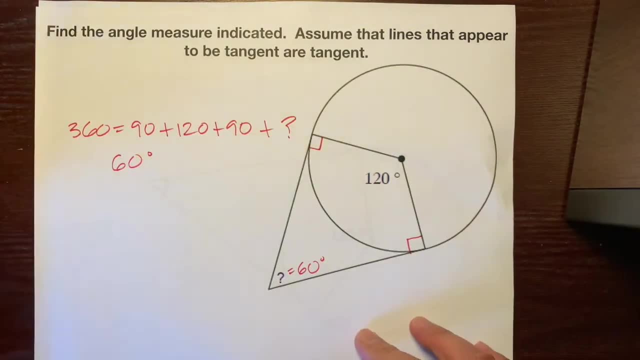 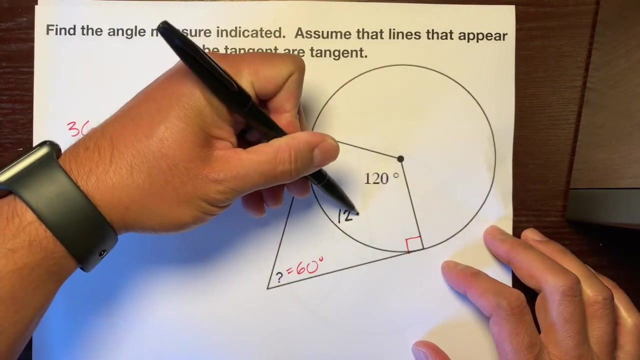 noticed, this is a central angle because the vertex is on the center, So that means that this arc is 120 degrees. I'm going to use a black pen because that's the only other color I have at the moment, and yeah. So this is 120 degrees right here and then the rest of this circle. so this 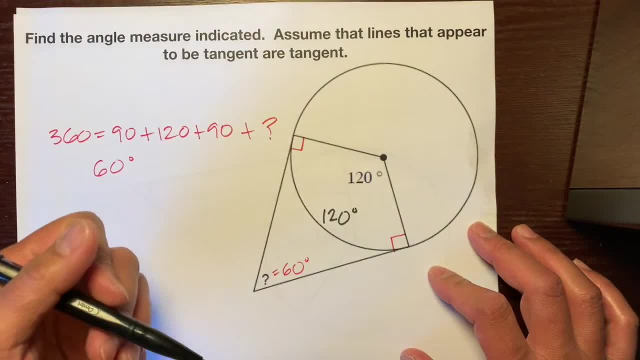 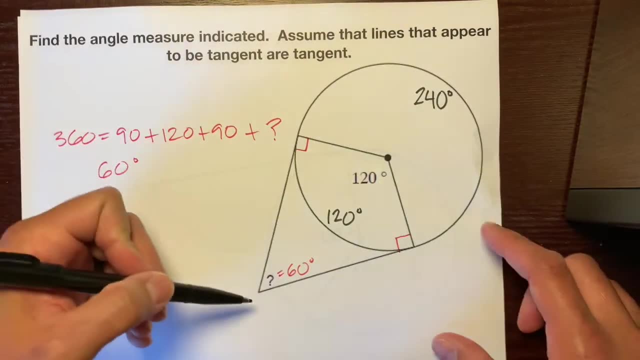 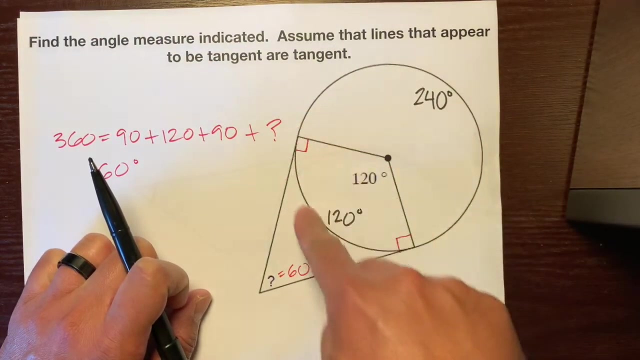 arc right here is 360 minus 120, so this would be 240 degrees. So what we could do here is take this arc, the far arc, subtract it from the near arc and divide it by 2, so we could do 220 degrees. 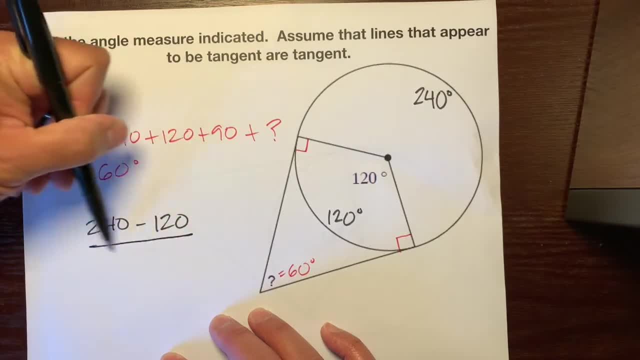 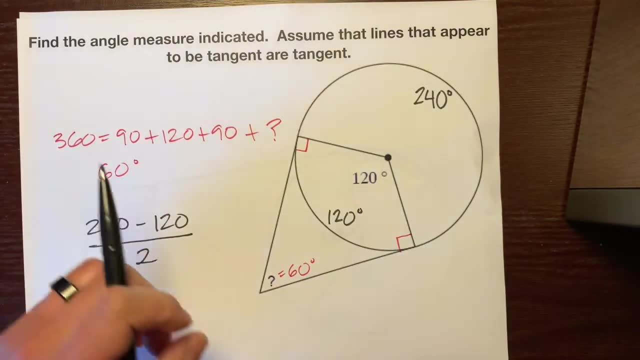 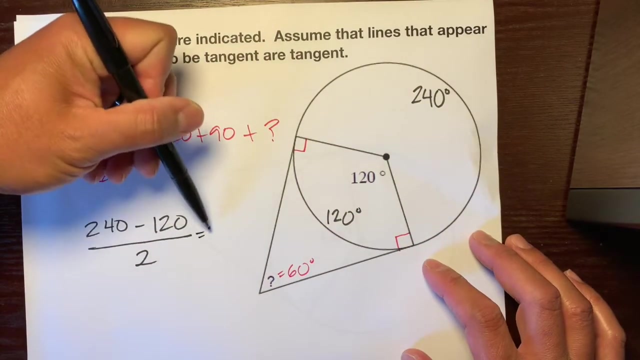 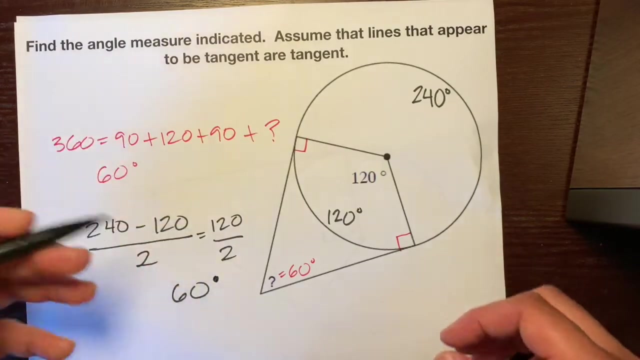 240 minus 120 divided by 2, because this angle intersects, or the angle's vertex is on the outside. So if you remember that concept, the far minus the near divided by 2.. So 240 minus 120 is 120 divided by 2.. Half of 120 is 60 degrees. So you can't just take this angle and divide it by 2. 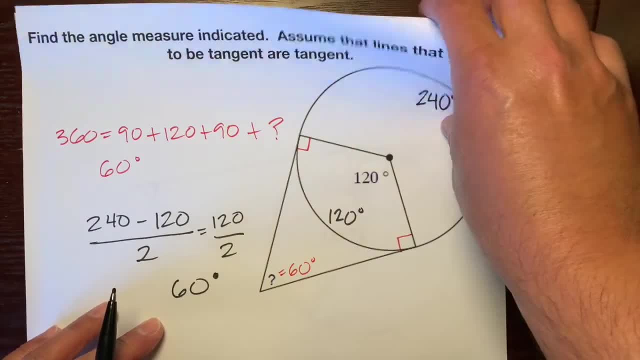 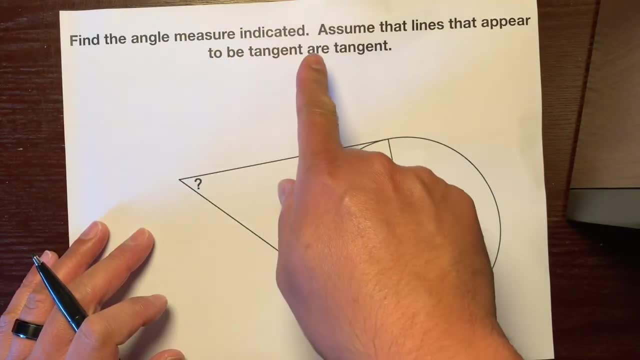 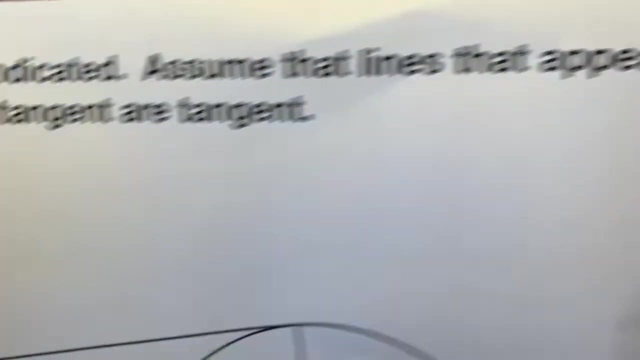 because it doesn't always work. So here's another example to prove that to you. So here it is. Same instructions. Find the angle measure indicated. So here's the indicated angle measure or angle. Assume that lines appear to be tangent or tangent. So if you remember,